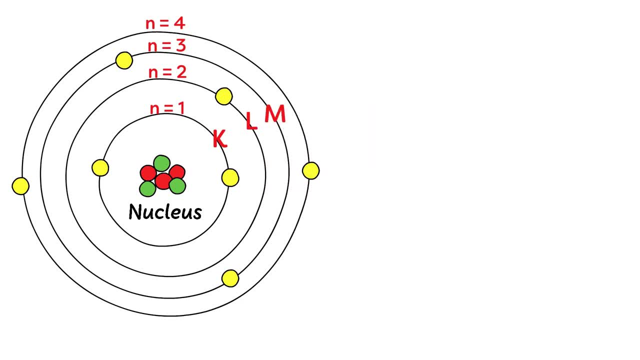 Third shell is known as a m shell and fourth shell is known as a n shell. To sum up this whole concept, we can write as-: when n is equal to 1, it is first shell, or k shell. when n is equal to 2. it is second shell or n is equal to 6th shell. When n is equal to 1, it is 1st shell, or k shell, iblok, and n is equal to 4 and m is equal to 5. to join in présent: slash belter. madrid IV- poles of interest. 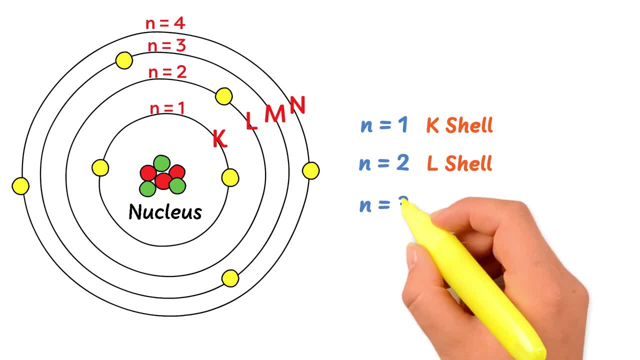 second shell or L shell. When n is equal to 3,, it is third shell, or M shell. When n is equal to 4,, it is fourth shell or N shell. Now pause the video and write it down. Secondly, every shell is divided into sub-shells or sub-energy levels. Sub-shells are denoted: 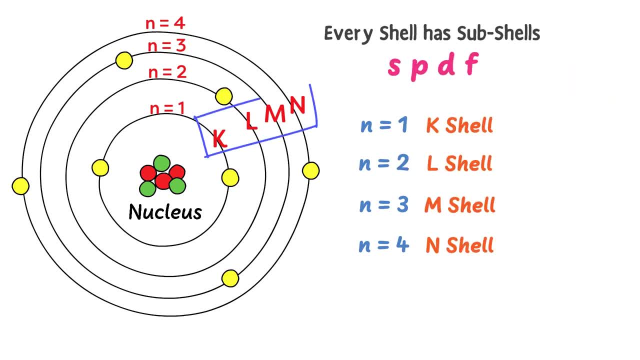 by SPD and F. So K, L, M and N are main shells, while SPDF are sub-shells within main shells. The first, or K, shell has only one sub-shell, S. The second, or L, shell has two sub-shells: S and P. The third, or M, shell has three sub-shells, S, P and D, While the fourth, or N, shell has 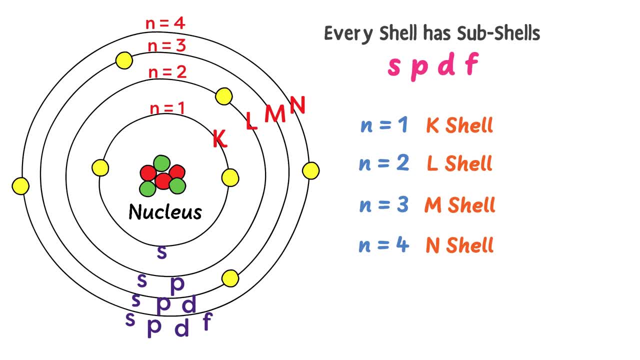 four sub-shells: S, P, D, F. The most easy trick to remember the sub-shells is: first shell has only one sub-shell, second shell has two sub-shells, third shell has three sub-shells and fourth shell has four sub-shells. Secondly, when you go from the first shell, 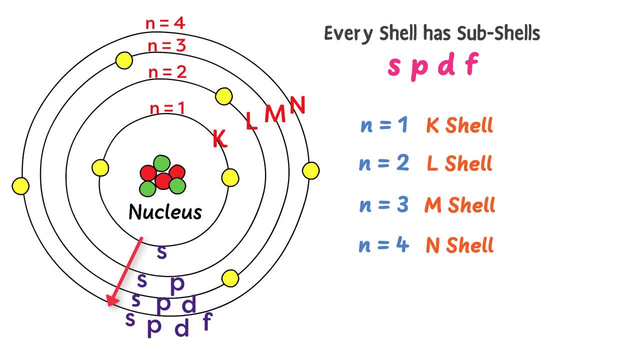 to the fourth shell. add one sub-shell successively like S, then SPDF, then L, M, N, N, F, L, P, then SPD and then SPDF. Now I write N is equal to one and we know that it is K shell. 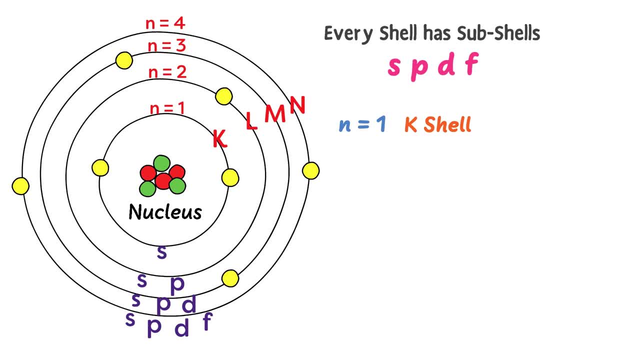 and K shell has only one sub-shell. I mean S Here. I write one with this S, because this S sub-shell belongs to first, our K shell. Secondly, N is equal to two. we know that it is L shell And there are two sub-shells. 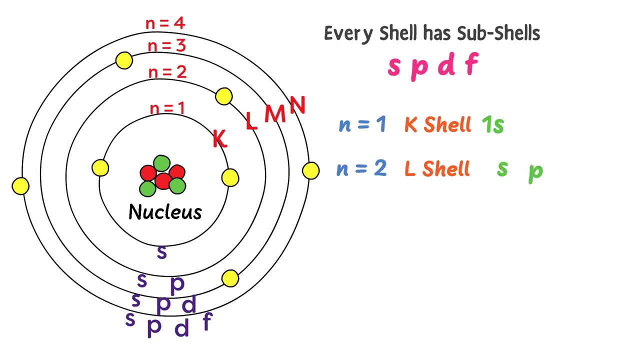 Sub-shell- Sub-shell- Sub-shell. Sub-shells N8,, S and P. I write two, with this S and with this P, because this S and P belong to second shell. Thirdly, I write: N is equal to three, It is M? shell and we. 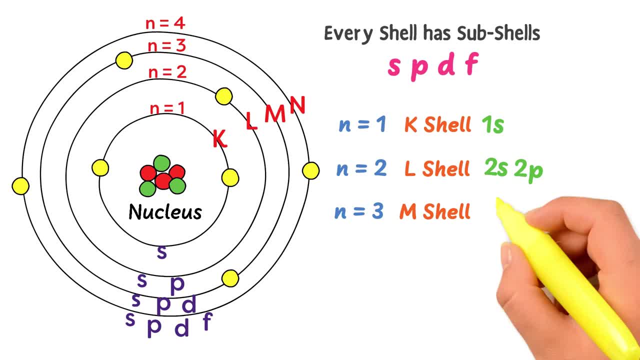 know that there are three sub-shells: N8, S P and D. I write three with S P and D because they belong to third shell. Fourthly, I write N is equal to four. It is N? shell and we know that it has four sub-shells. 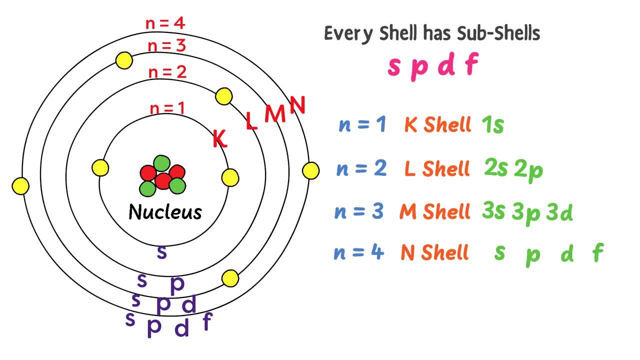 S, P, D and F. I write four with S, P, D and F because they all belong to fourth shell. So if I write three S and four S here, can you guess the difference between them? Well, three means third shell and F. 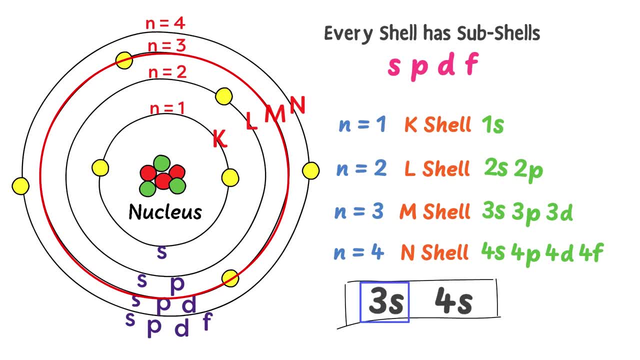 S means sub-shell. So three S means S is the sub-shell of the third man-shell, our M shell. Similarly, four S means S is the sub-shell of fourth shell, our N shell. Finally, let me teach you that what are orbitals? 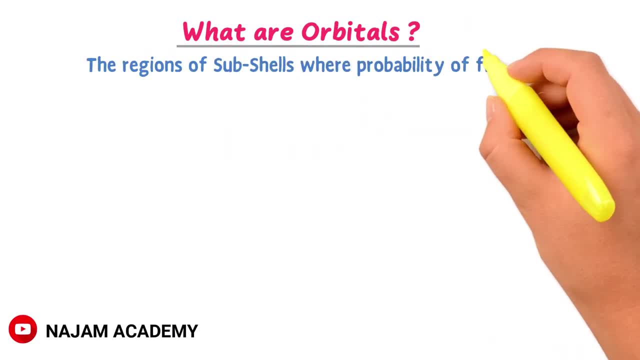 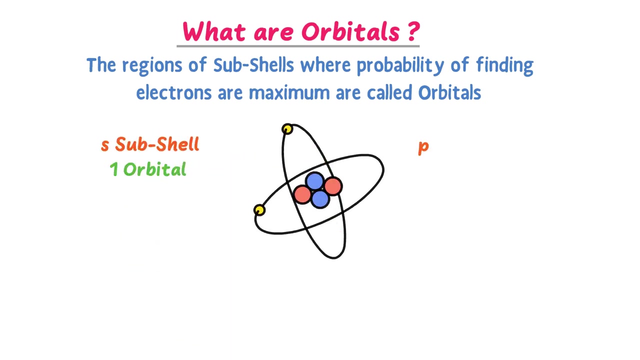 Well, the regions of sub-shells where probability of finding electrons is maximum. These regions are called orbitals. You can say that these are the three-dimensional paths where chances of finding electrons are maximum. For example, S sub-shell has one orbital, P sub-shell has three orbitals and D sub-shell. 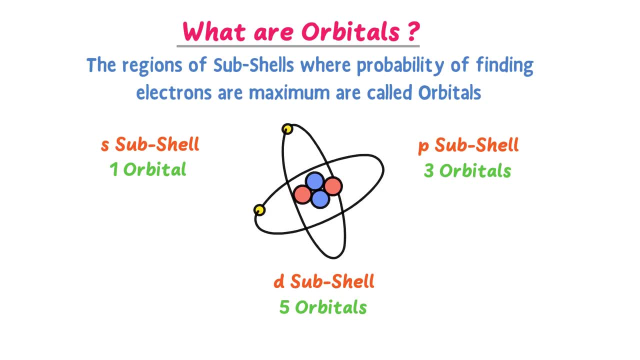 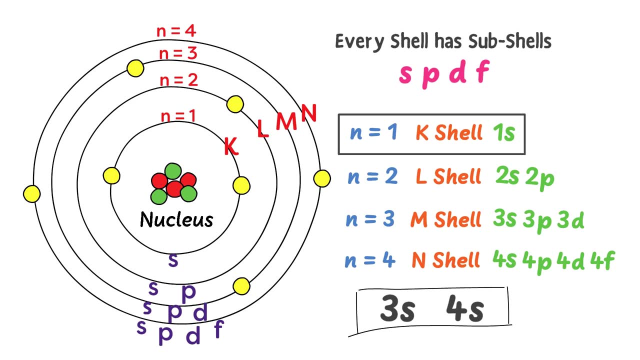 has five orbitals. To summarize my lecture, we learned that there are different shells around the nucleus, like when N is equal to one, it is K-shell and it has one sub-shell, 1S. When n is equal to two, it is L-shell and it has two sub-shells, 2S and 2P. 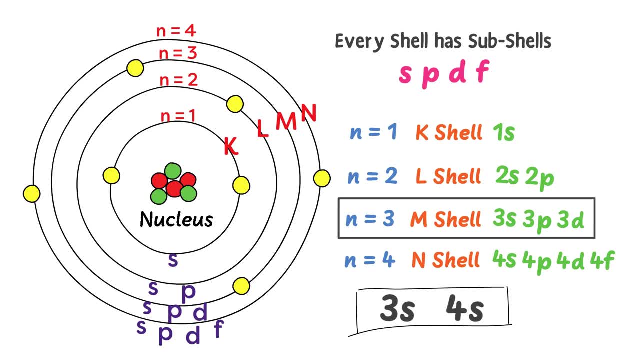 When n is equal to three, it is M shell and it has three sub-shells: 3S, 3P and 3D. When n is equal to four, it is N shell and it has four. You can see that this is a two-dimensional path. 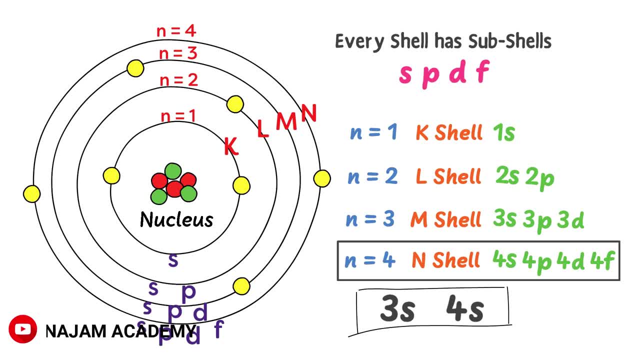 It has four sub-shells: 4S, 4P, 4D and 4F. This was all about shells, sub-shells and orbitals. 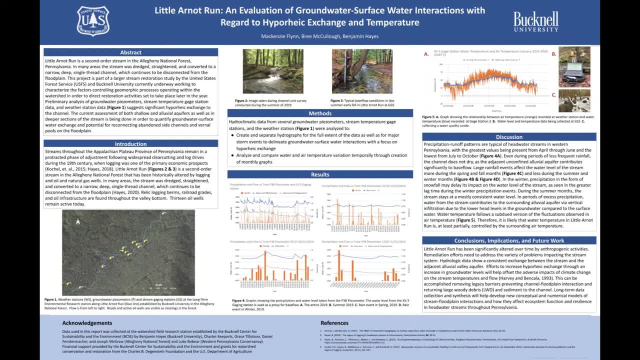 Our project consists of an evaluation of groundwater-surface water interactions with regard to hypereic exchange in temperature in Little Arnett Run, a second-order stream in the Allegheny National Forest that has been historically altered In many areas. the stream was dredged, straightened and converted to a narrow, deep, single-thread channel, which continues to be disconnected from the floodplain. 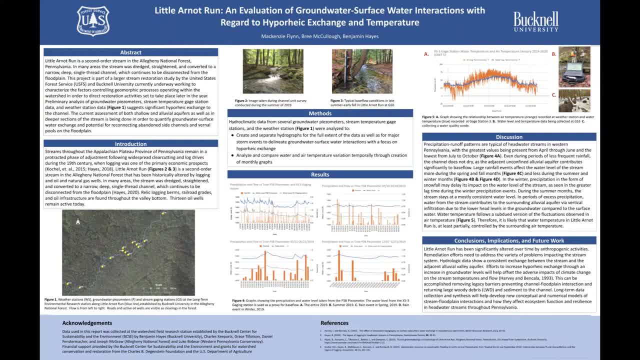 This project is part of a larger stream restoration study conducted by the US Forest Service and Bucknell University that's working to characterize the factors controlling geomorphic processes operating within the watershed, in order to direct restoration activities set to take place later in the year. 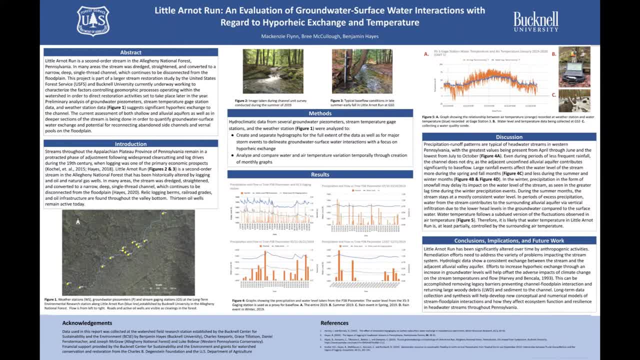 Preliminary analysis of data suggests significant hypereic exchange to the channel. This data was further analyzed to create a series of hydrographs to delineate the groundwater-surface water interactions, with a focus on hypereic exchange. It was also utilized to analyze the flow of water. 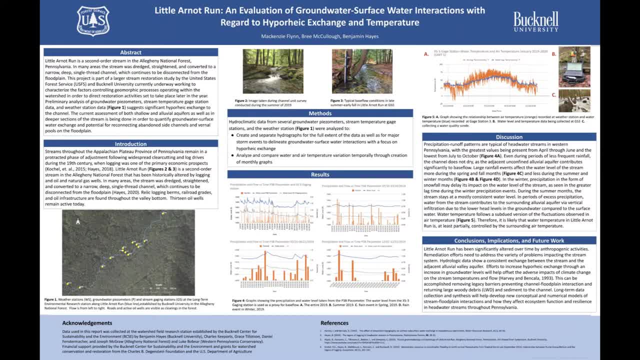 Let's analyze and compare water and air temperature variation temporally. The rainfall displayed in the data is typical of Pennsylvania. During drier periods, the channel does not dry due to the adjacent unconfined alluvial aquifer contributing to base flow.